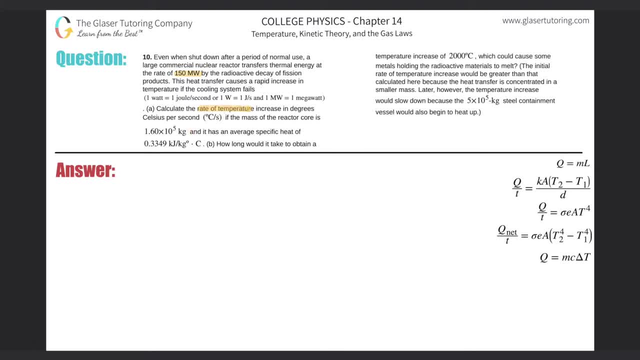 Letter A. Calculate the rate of temperature increase in degrees Celsius per second if the mass of the reactor core is 1.6 times 10 to the 5 kilograms and it has an average specific heat of 0.3349 kilojoules per kilogram Celsius. 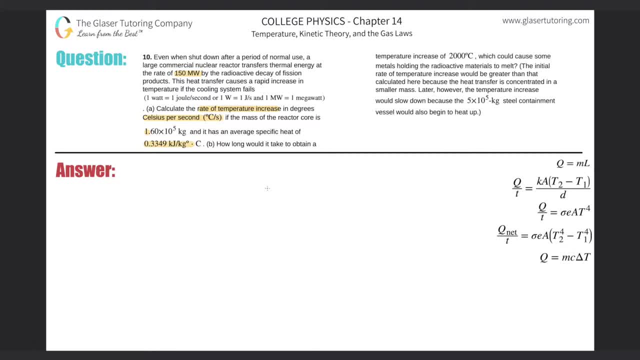 All right. So first thing is, it sounds. I mean it doesn't. it definitely sounds like it, right. I mean, they're giving us mass, they're giving us a specific heat here, So more than likely, we're going to be using this formula. 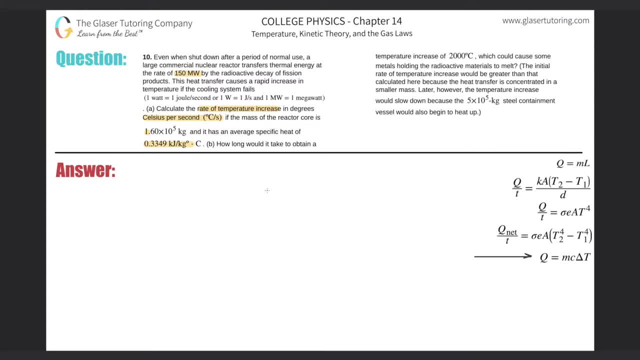 But I know the problem that you might be thinking. you might be saying: well, that's great, I mean, I can calculate temperature, but we don't know the, just the energy, right, We know the power. Now I can make one adjustment to that equation so that we can substitute in power instead of just energy. 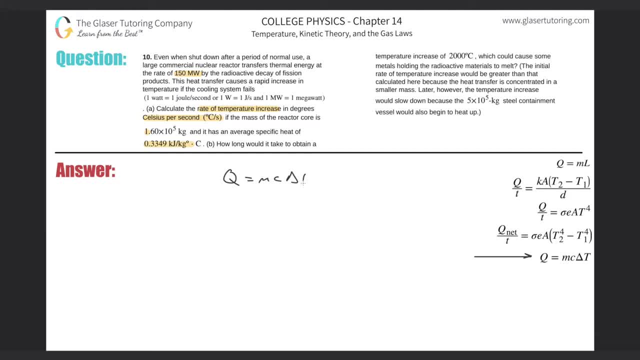 Watch. So here we have: Q is equal to MC delta T. Now you know with the rules of math that whatever I do to one side of the equation, I should always I should also do to the other side of the equation. So if I were to divide this side by, let's say, seconds aka time, then I would also have to divide this side by time. 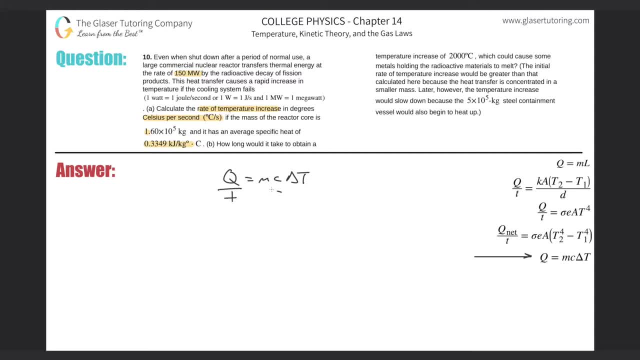 Now, if I do that, watch what happens. I put this over T and then I put this over T. Now, the key insight here is that energy per time- right here, energy per time is power. That is the definition of power. Recall that power is equal to energy over time. 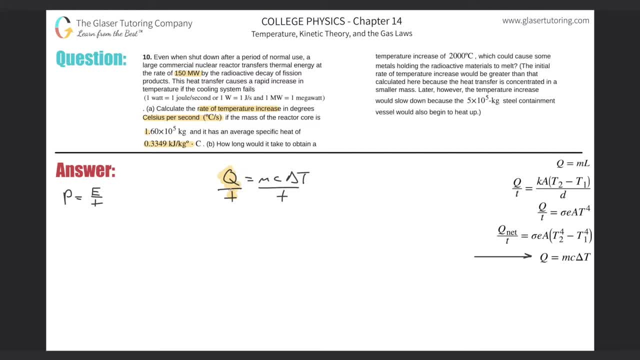 Now I know that it's Q here. The only reason why it's Q is because it's heat energy. But energy is energy. So I mean there's different forms of energy. I mean, you know what I mean. So in this particular case we can now call this: power is now equal to mass times, specific heat times, change in temperature, all divided by the time. 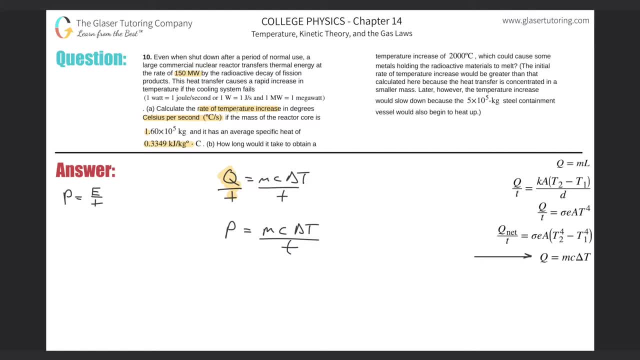 Now what, What, What we are after again, we are after calculating the temperature increase in degrees Celsius right per second. So basically I want to now find this temperature per time. So my goal here is to solve now this equation for capital T over lowercase T, meaning temperature per unit time. 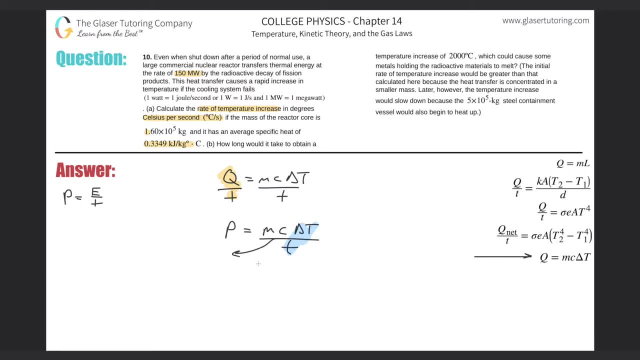 So I'm going to bring then the mass and the specific heat on over to the left-hand side, right, by dividing it out. So it's going to be the power divided. by then, the mass multiplied by the specific heat will equal now the change in temperature per time or the rate of temperature change, right? 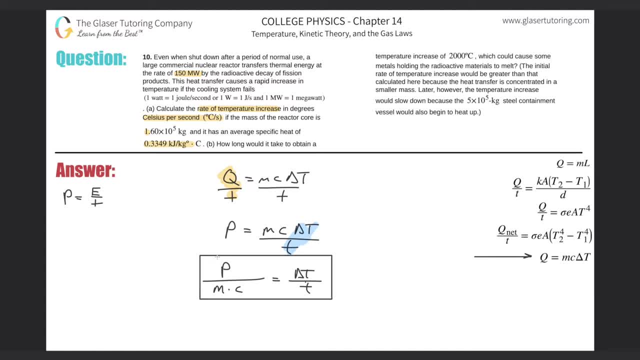 And lo and behold, problem's simple. It's simple now, right? It's very simple. So now all we have to do is plug in. Now, just remember: you've got to make sure you have the right units, All right. 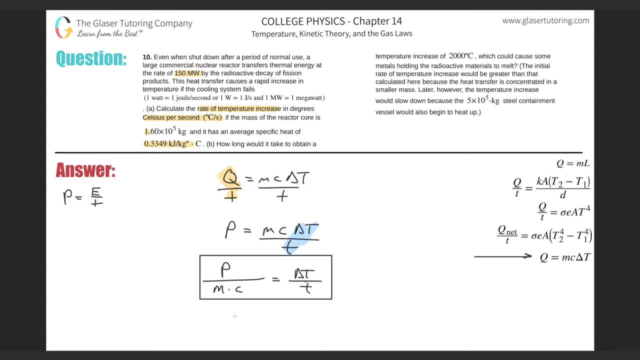 So they gave it to us in megawatts, but we need it in watts, So just multiply that value by 10 to the sixth. Okay, so it's going to be 150 times 10 to the sixth. Going through the convergence quickly here, because they should be good at this point. 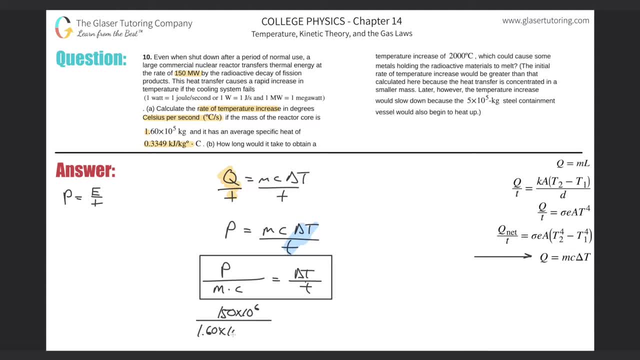 The mass here is 1.60 times 10 to the fifth kilograms. That's the appropriate unit. And then- just be careful with this- All the units are correct, except for the kilojoule right. We'd like to have that in joule. 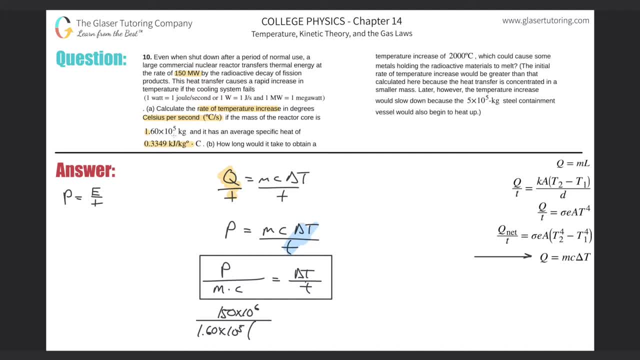 And what I'm going to do then is basically I have to then Multiply that, excuse me- by 1,000.. All right, So now that's going to be 334.9.. Don't know why that took me so long. 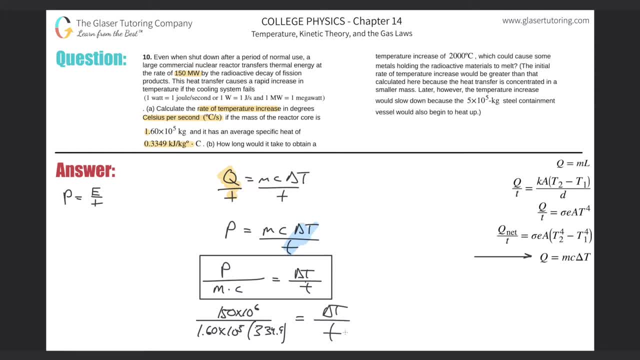 It's a little early, I think, And I didn't get too much sleep last night. What are you going to do? So here it is, guys. All right, Now all we have to do is just plug it on into the calculator. 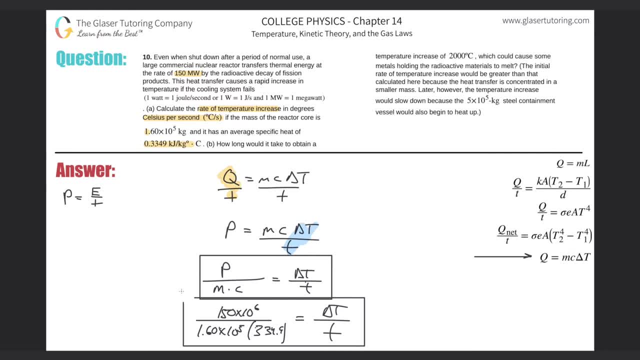 Okay, All right. So 150 times 10 to the sixth, Divided by then parenthesis, 1.6 times 10 to the fifth, Multiplied then by 334.9.. And here we get about So every second, And this is pretty fast. 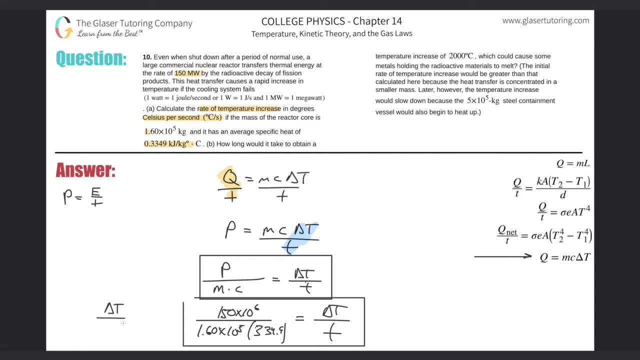 So every second the temperature will be changing by a value of 2.8, or so 2.99,, 2.80.. 2.80,, I guess, with sig figs, Degrees Celsius, Degrees Celsius, So that doesn't take long for it to overheat, right. 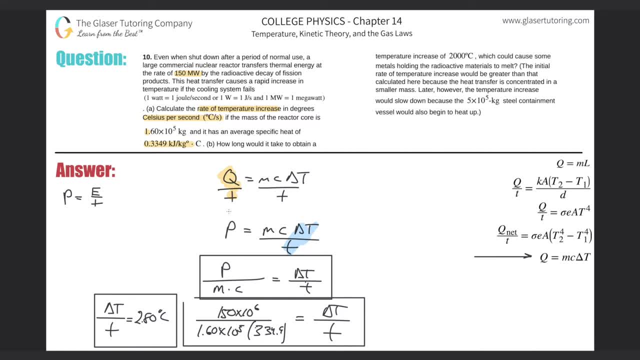 10 seconds, That's 28 degrees Celsius. 100 seconds- Right, That's 280 degrees Celsius. 100 seconds isn't even two minutes. So you can kind of see how this can get out of control quite quickly, Anyway.